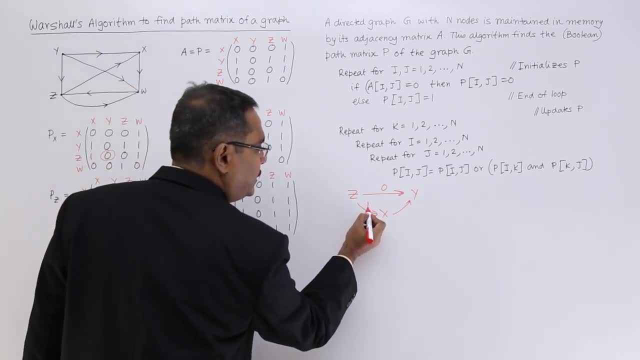 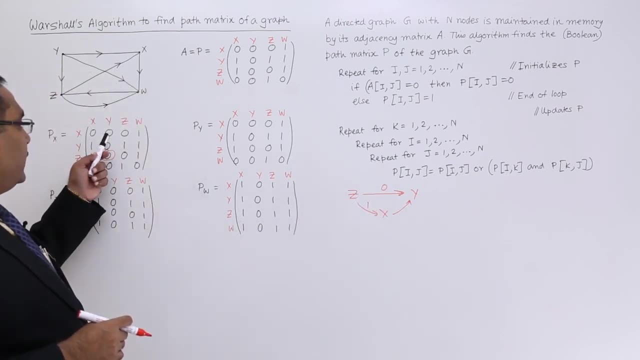 So Z to X is 1.. So I am highly optimistic that we are going to get another parallel path. But from X to Y you are getting 0. So if you take the AND it is 0,, 1 AND 0. 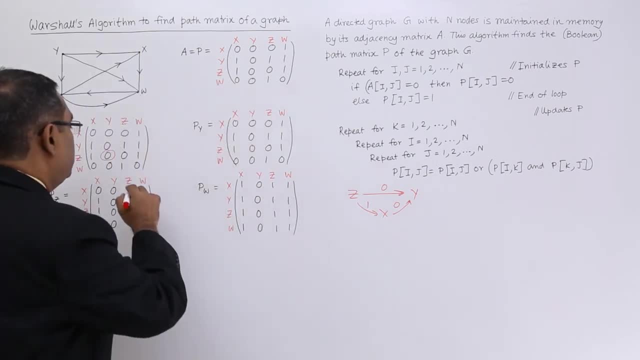 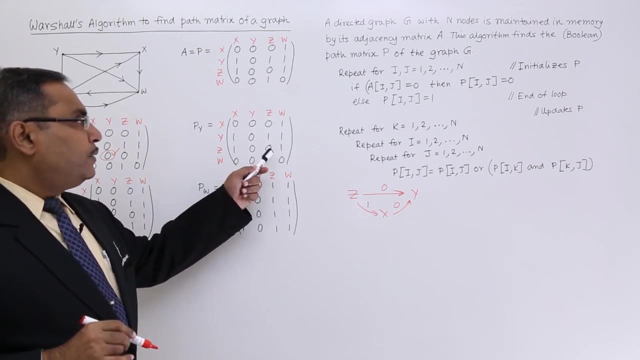 equal to 0 and 0, or 0 is equal to 0. So that is why this value is still with 0.. Similarly, taking this y as intermediate, we have formed this one. always remember: from here we are forming this. from here we are forming this. from here we are forming this. 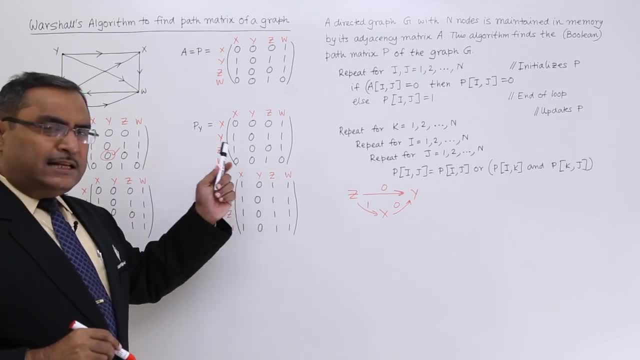 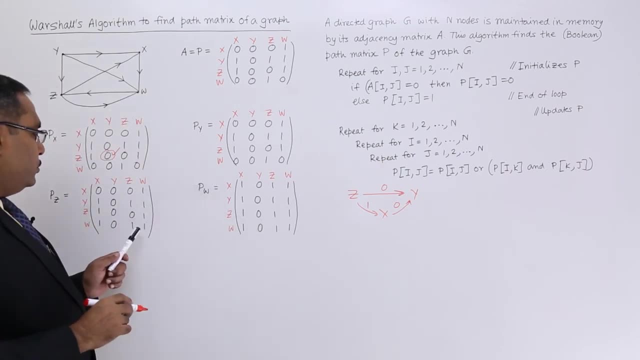 and from here we are forming this So that the last contribution will remain, survive there. Now see, so let us consider this one. I am observing one change here. I am observing one change. I am considering this one. What is this? That is w w so. that is a w w So. 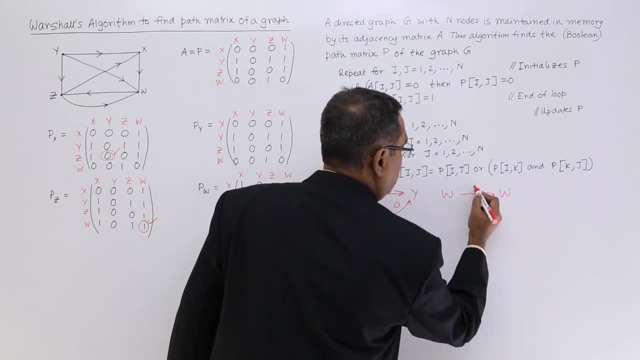 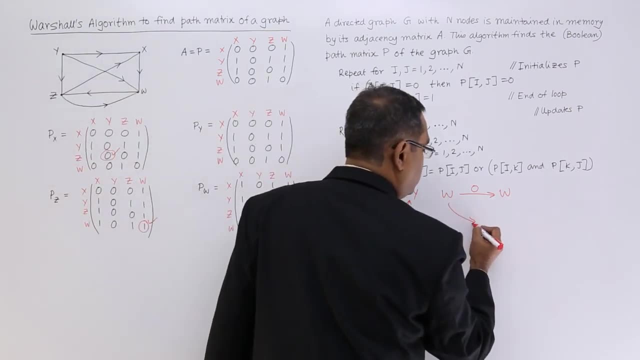 from w w. we are having no path. Now, what is the intermediate one Here? intermediate one is z, intermediate one is z. So I am coming to z and z to w. So let me, let me check. so w to z. 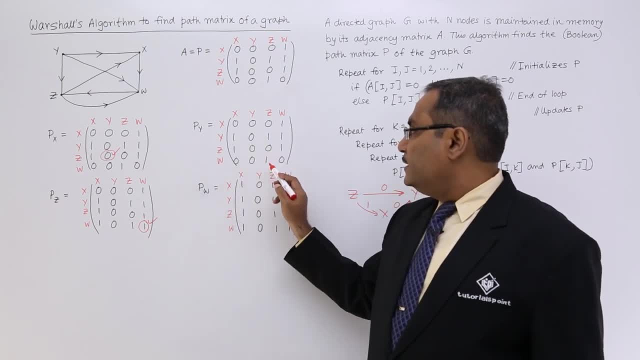 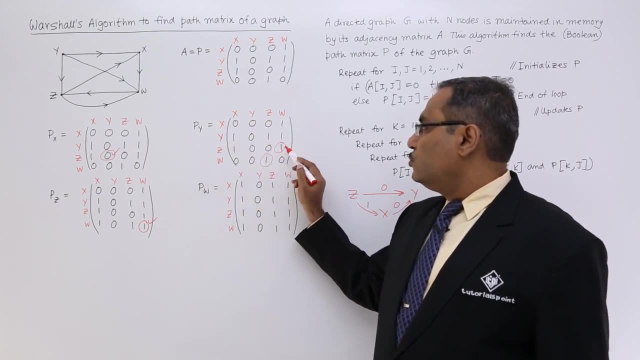 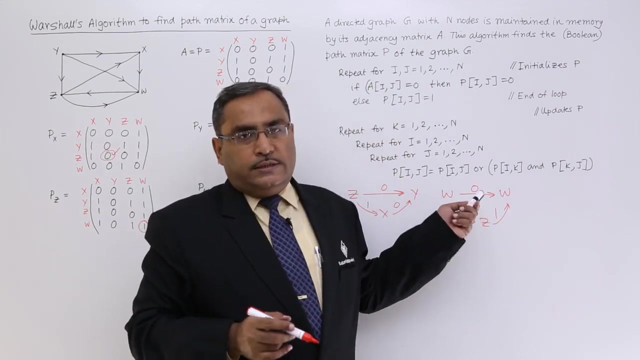 For this one. so w to z is 1 and z to w, z to w is also 1.. So 1: 1.. So now just go for 1, 1.. So 1 and 1 is 1, and 1 or 0 is equal to 1.. So that is why w, w this cell is having. 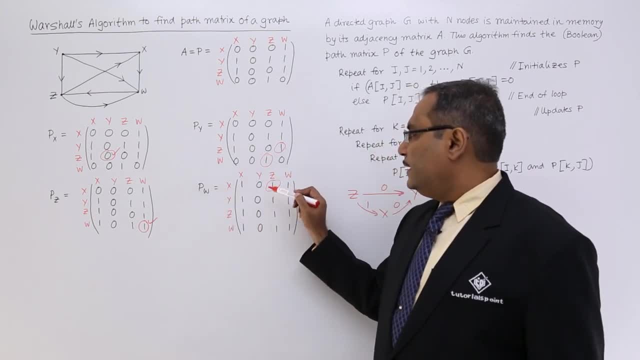 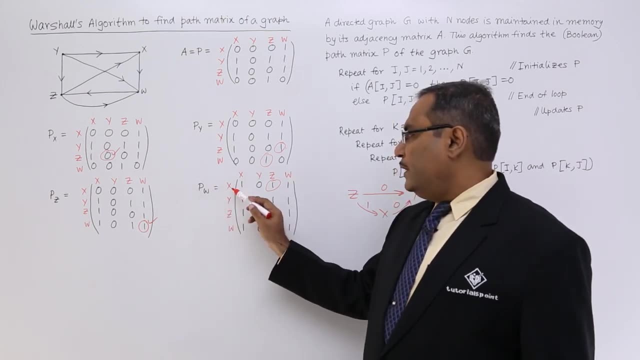 the value 1.. So just consider this one now. take this one as an example. So what is the intermediate node here? True node, that is a w. So x to z, x to z. initially x to z is 0. So that is no path. Now, please, 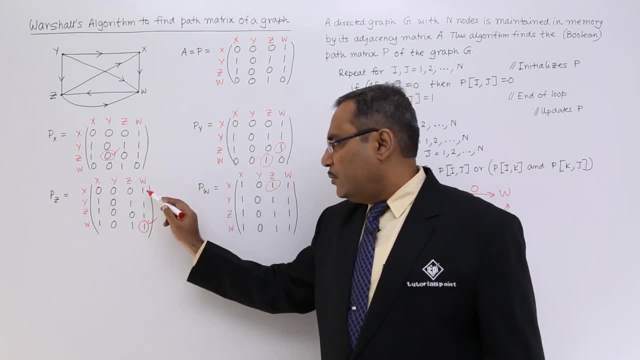 come through w, x to w, So x to w is 1.. So I am highly optimistic and then I am going for. I am going for w to z, So w to z is 1.. So it indicates that it will be 1.. So this: 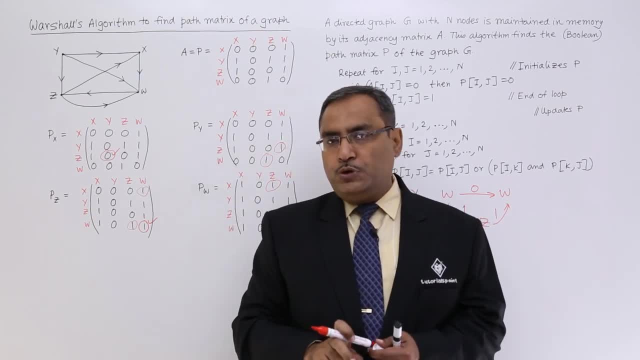 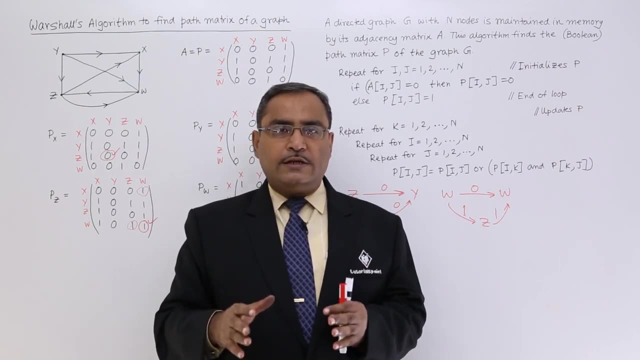 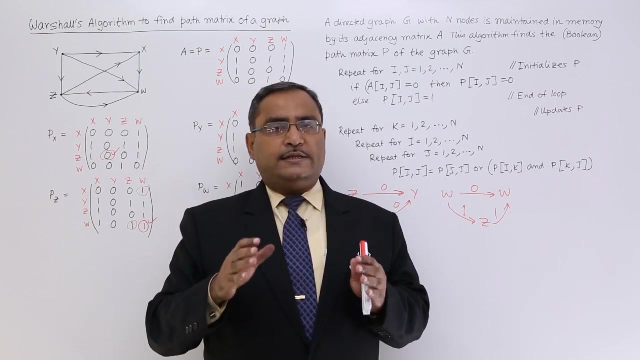 is my final path matrix and that is the output, that is the return from this Warshaws algorithm. So in this way, Warshaws algorithm can find the path matrix from the graphs, adjacency matrix. So now I think the algorithm is clear to you and this particular example has cleared.